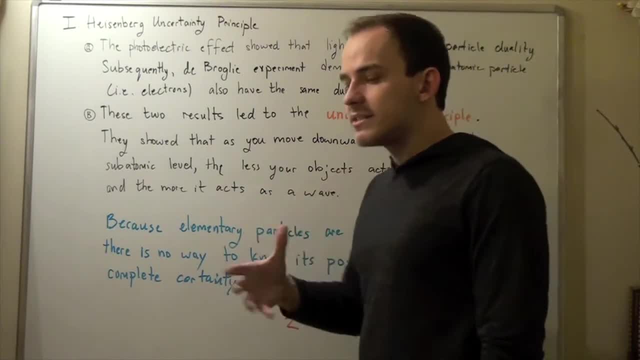 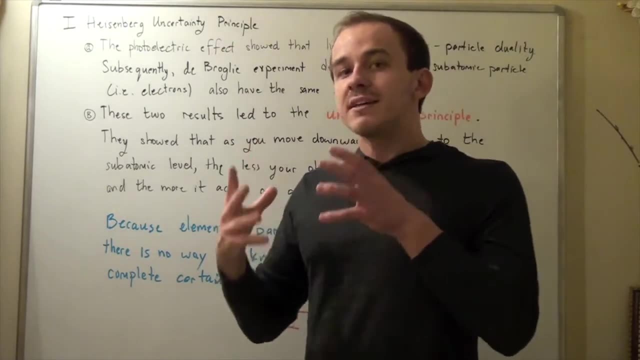 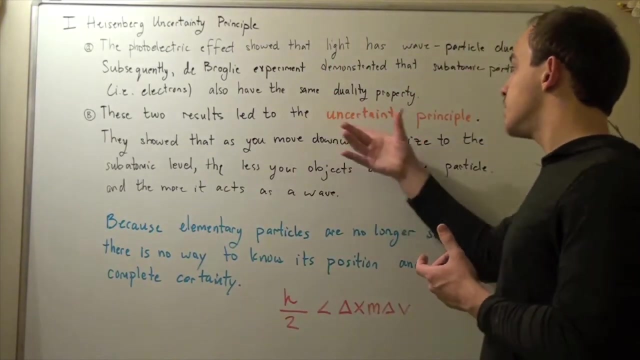 as a wave. In other words, as you get down to the subatomic level- see the electrons and protons and neutrons electrons- the less your objects act as solid spheres and the more your objects act as waves. Now, to demonstrate what this uncertainty principle states, I'll use the following example. 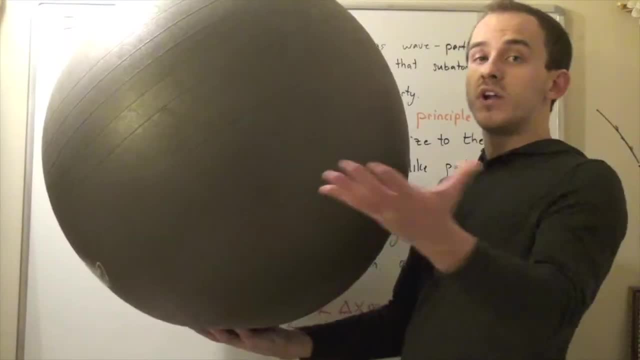 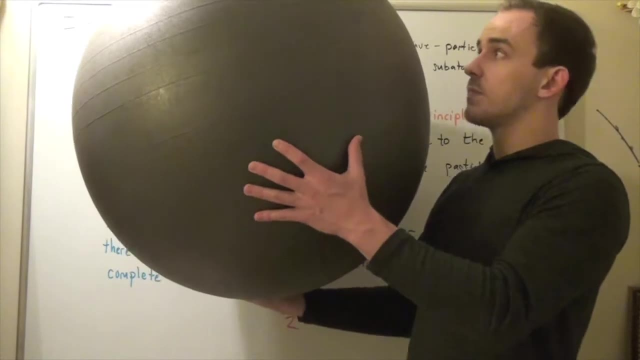 Suppose I have this relatively large ball which from where you're sitting you can probably tell where the ball is, and you can tell the ball isn't moving, so you can tell its velocity. Now suppose I go smaller. Suppose I hold up this ball. Now, once again, this is a relatively 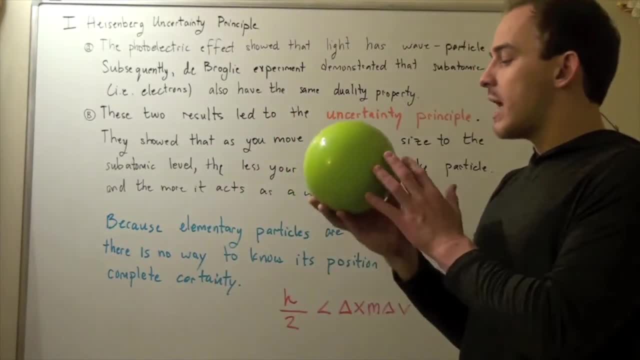 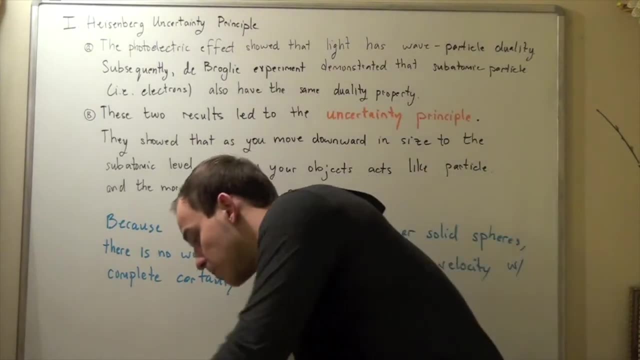 large ball and from where you're sitting you can probably tell that the ball isn't moving. and you can tell where the ball is. Now suppose I go even smaller. Suppose I go down to this really tiny marble which you probably can't see from where you're sitting, but I'll move it. 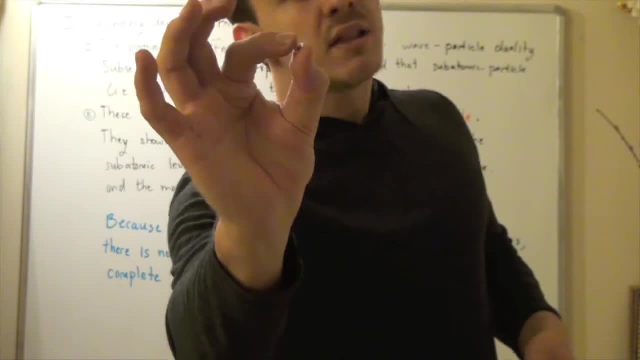 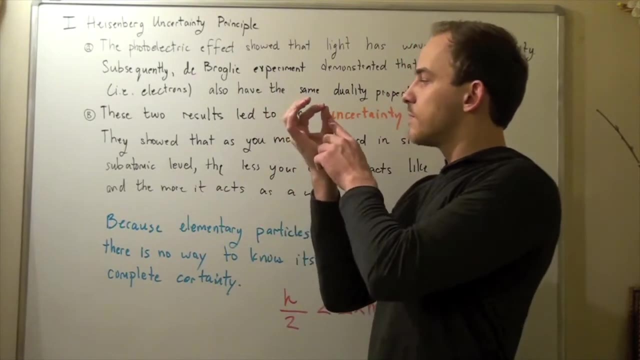 closer. Now there's my particle, There's my solid sphere. Now, now that you saw the sphere, you could probably see that. you know, you could probably see it from where you're sitting. But suppose now I walk a mile away or a kilometer away, and suppose I hold this. 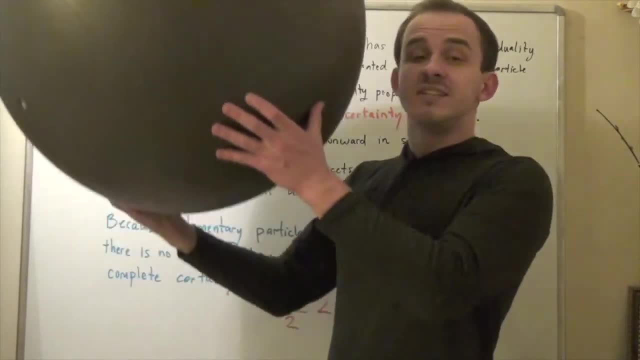 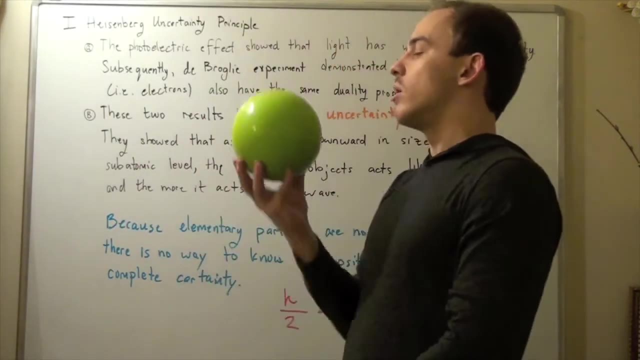 ball now. Now this ball becomes a speck. You could still see it, but it's much, much smaller. Now suppose I walk a mile away and I hold this ball up. Now, this ball you probably won't see really well. You might see it if you have really good vision. but 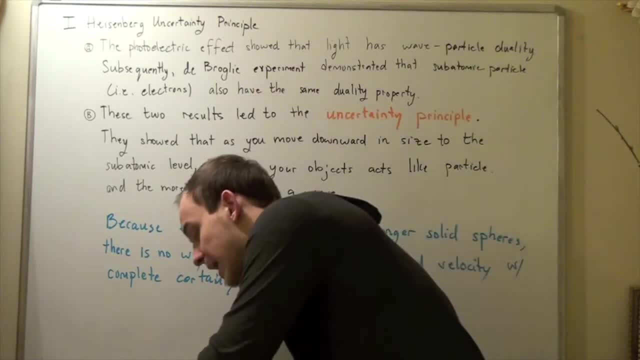 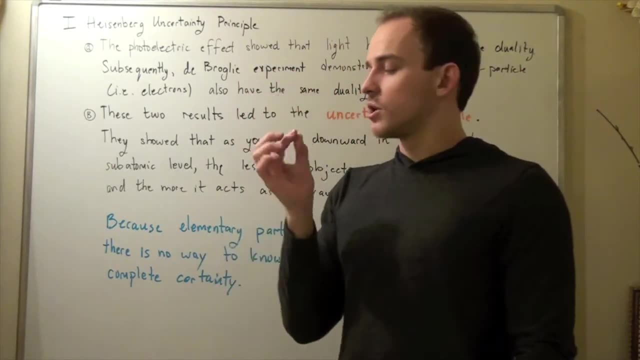 I don't think I'll see it a mile away. Now suppose I hold this really tiny marble, the solid sphere, from a mile away. You definitely won't see this one right? So in other words, the smaller you go, the less you see its position. 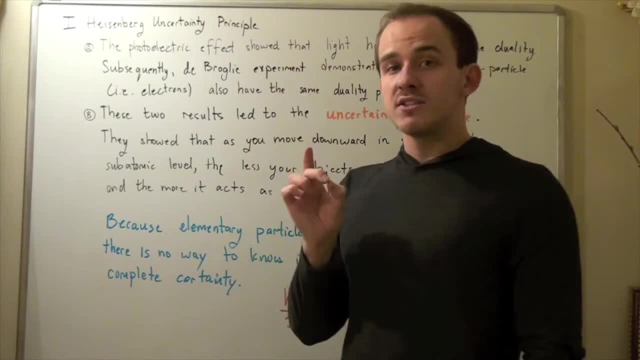 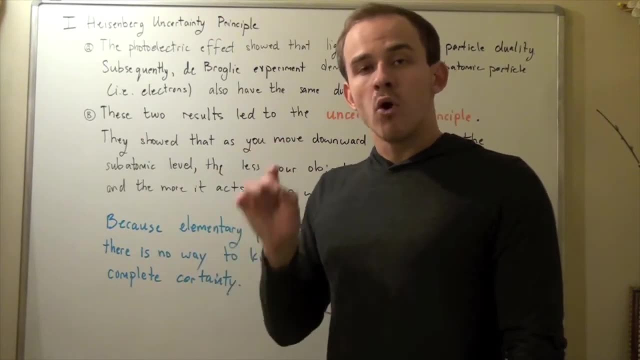 and the less you see its velocity. If I walk five miles away and I hold either of these balls, you won't see any ball and you can't, and you won't be able to tell where the ball is and with what speed or with what velocity it's moving. Now the point is: and what's? 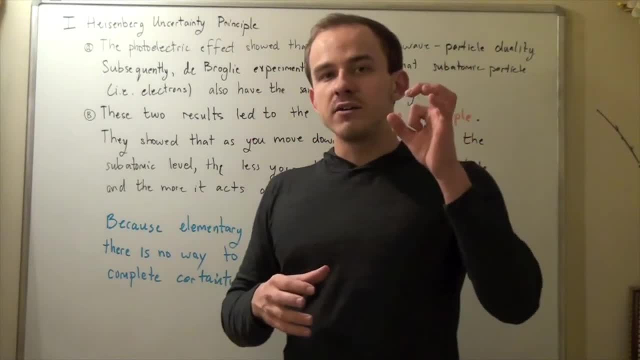 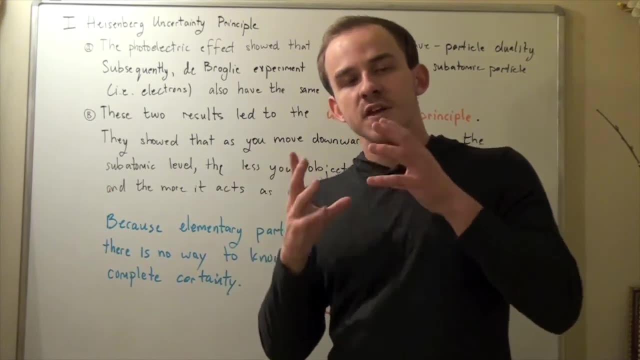 this uncertainty principle show is that as you shrink down to the atom and then to the sub-atom, to the electron, you no longer are dealing with solid spheres. They're no longer solid spheres and they act more as waves, In other words, they have both wavelike. 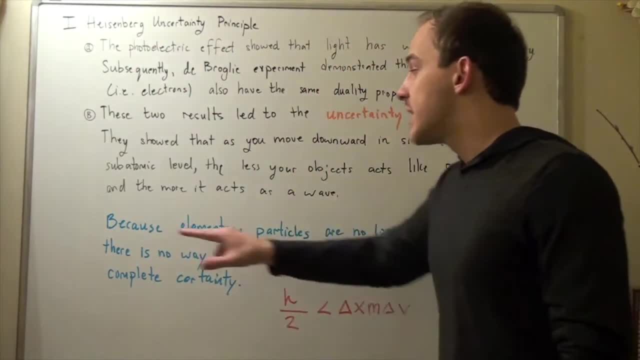 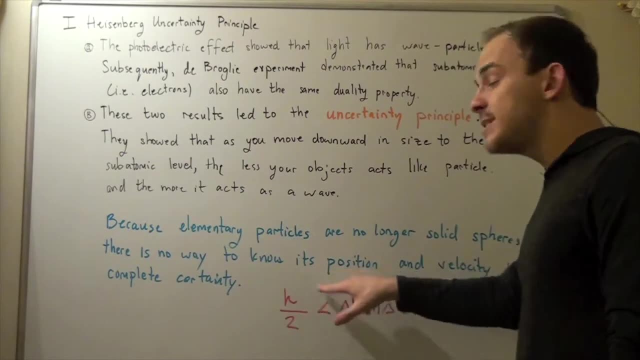 properties and solid properties. And that means, because elementary particles are no longer solid spheres, there's no way to know its position and at the same time its velocity. So again, you have to understand that the more you hit something, the more you crack. 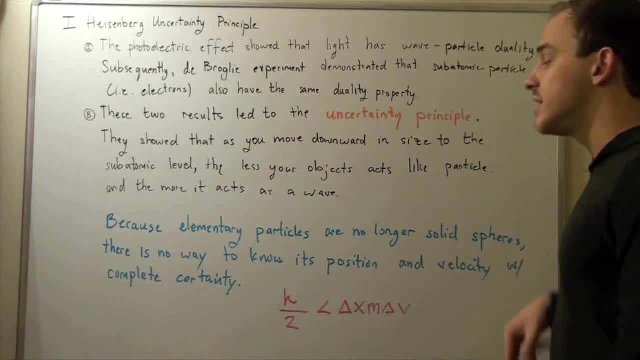 this small particle, the more you can think about it. In other words, when you run up, you see the difference in the amount of weight of the ball, and the more you count them in its velocity with complete certainty. So the formula or the equation for this uncertainty? 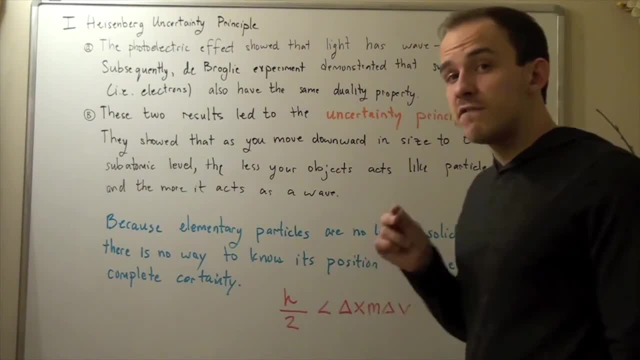 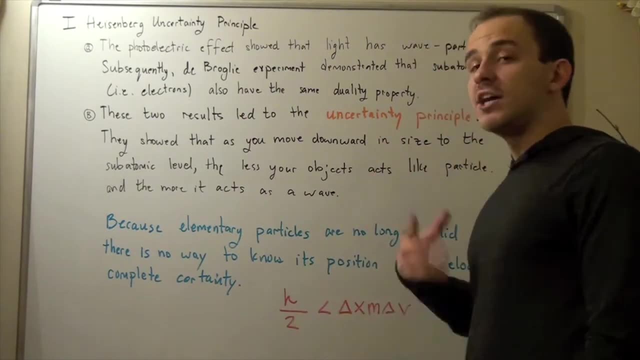 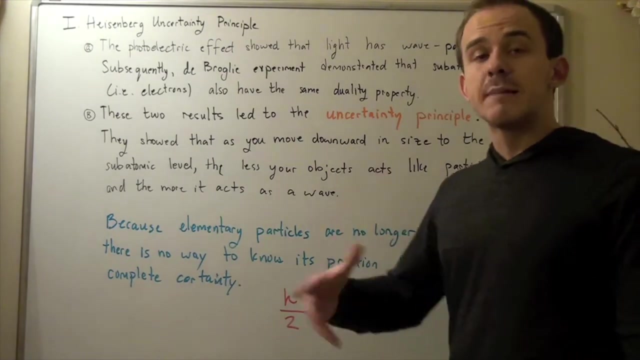 principle is the following: Planck's constant, a very, very small number divided by 2, is always less than our change in x or the uncertainty of our position. change in position times, mass times. change in velocity. Now remember mass times, velocity is momentum, So this guy is change in. 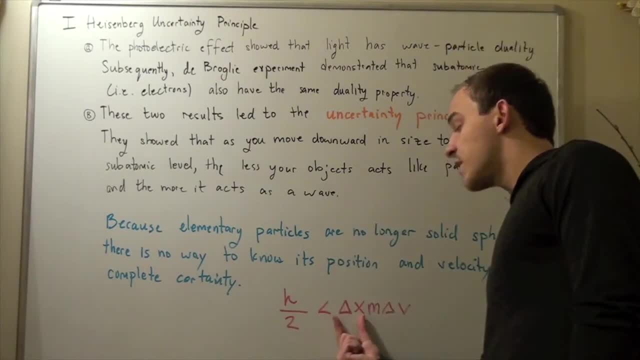 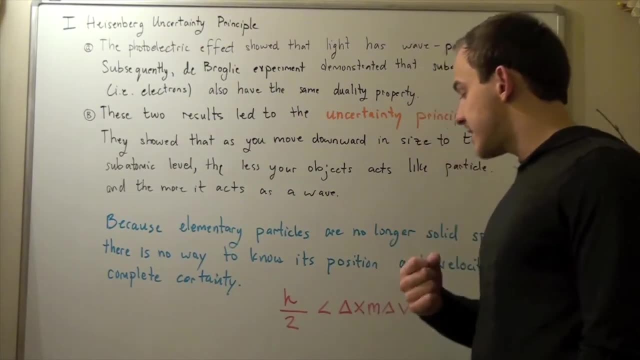 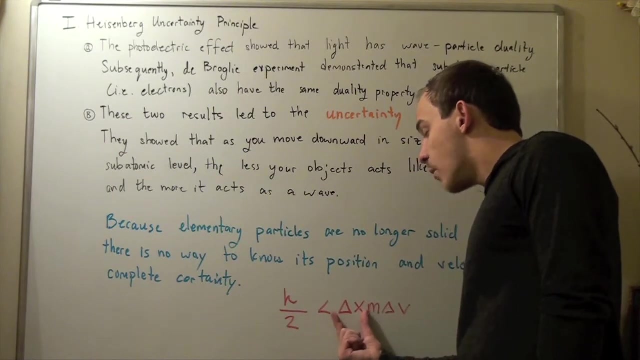 momentum. In other words, this is the uncertainty of our position and this is the uncertainty of our momentum or velocity. And what this equation basically says is the following: The less our change in x is if this guy is very small, that means we know more information about our position. 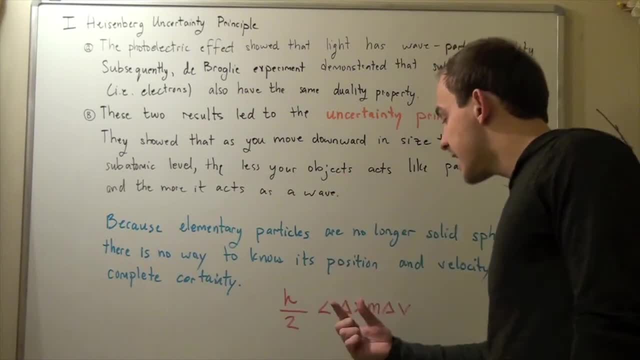 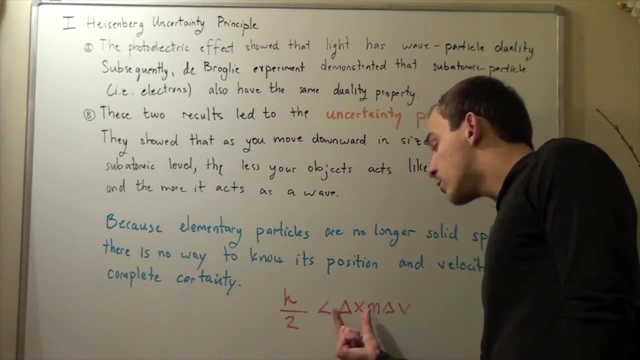 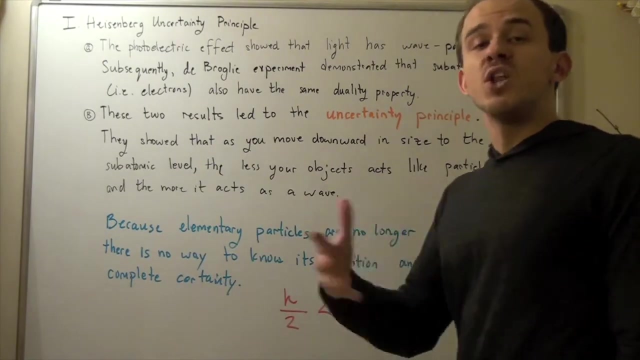 where our electron is located. And that means if this guy decreases- and this is a constant, this guy is a constant- must increase. The smaller our change in x is, the more we know about our position. the greater our change in v is, the less we know about our velocity, And likewise. 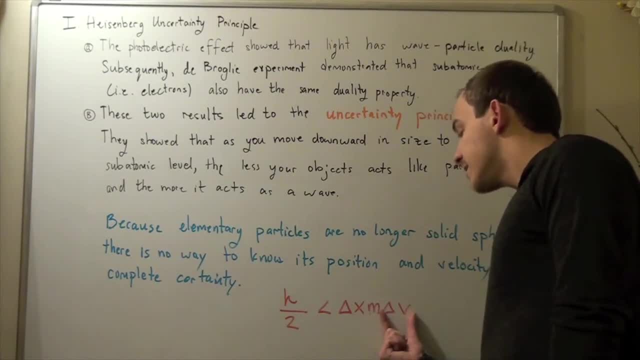 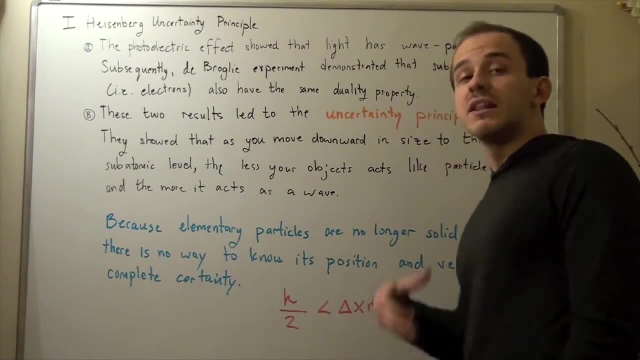 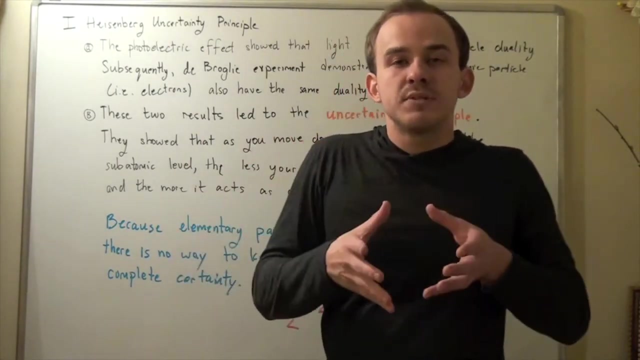 the same holds: The more we know about our velocity, change in velocity, the less our change in velocity is. and the less we know about our change in x, the less we know about our position. In other words, we can't be very certain about our position and at the same. 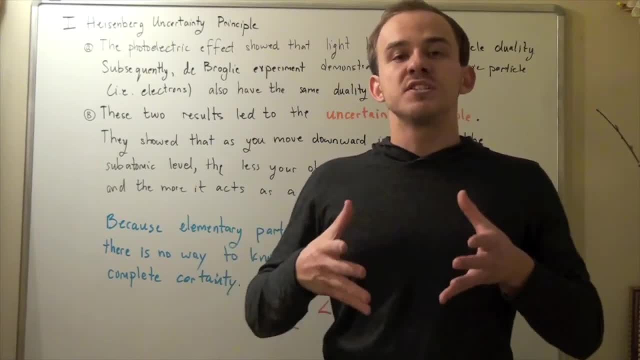 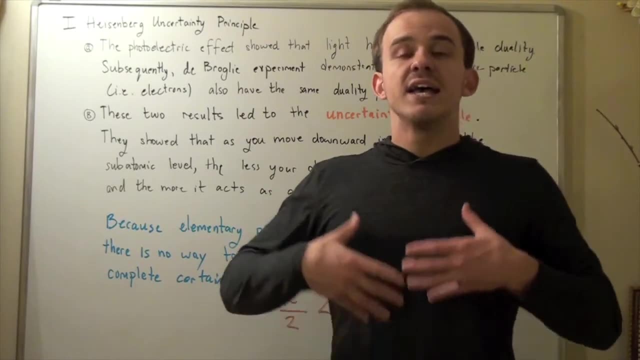 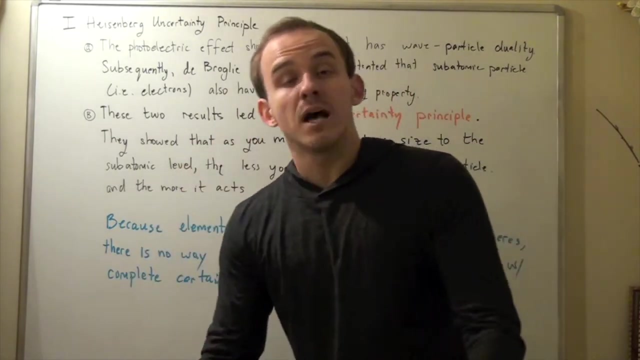 about our velocity. That's what the uncertainty principle tells us, And this has to do with the duality nature of subatomic particles, electrons and protons, as well as the duality of light. In other words, when you go from a large ball, from this ball to a subatomic particle, our 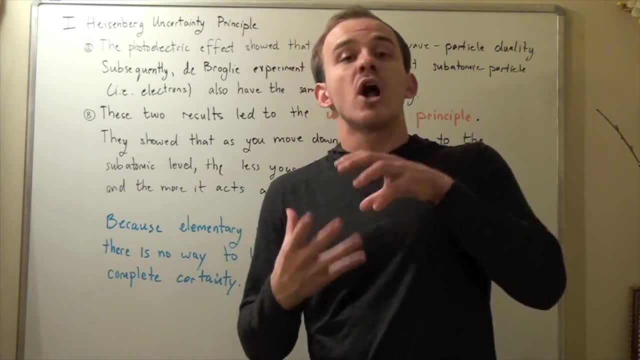 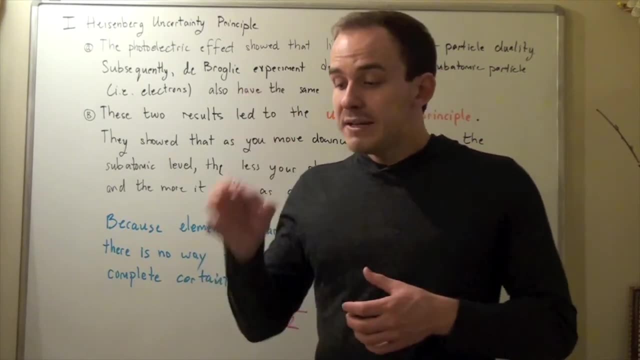 particle loses its solid sphere-like properties, It stops acting like a solid sphere and starts acting more like a wave, And therefore we can no longer be very certain about our velocity. We can no longer pinpoint exactly where our object is and at the same time,